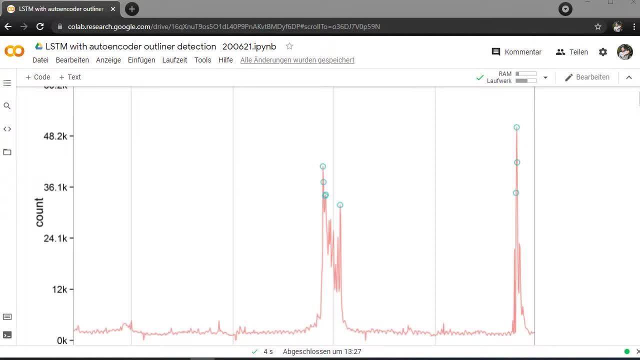 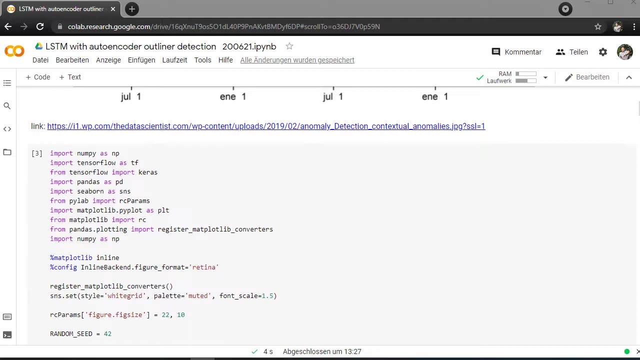 And then you can find these outliners here Rapidly increasing in the signal. This is what the outliners are basically. They are not normal due to the normal signal distribution. So to just check the code, here we start. first of all, 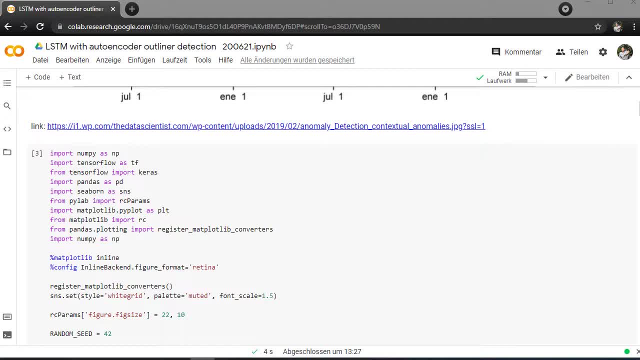 And if you like this channel, of course, subscribe, Hit the like button And I would be really happy about it to see you in the next tutorials. So in the first section here I inserted all the libraries that are necessary for this outliner detection. 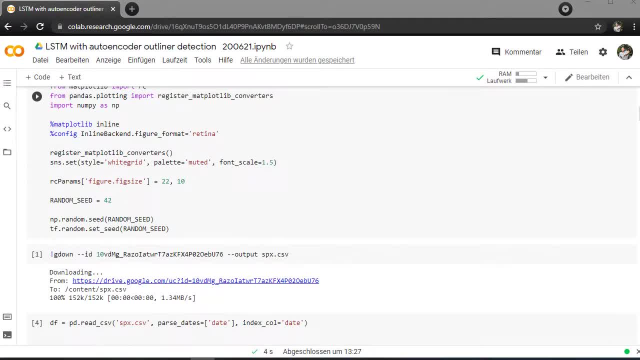 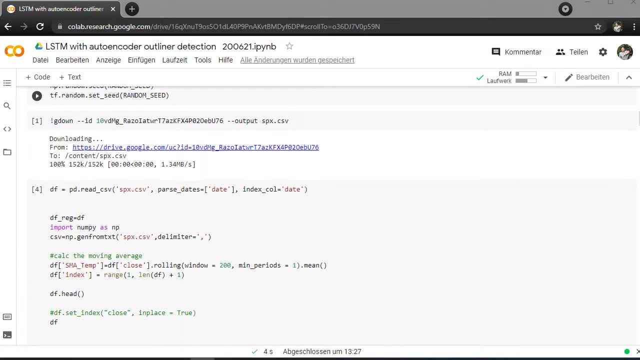 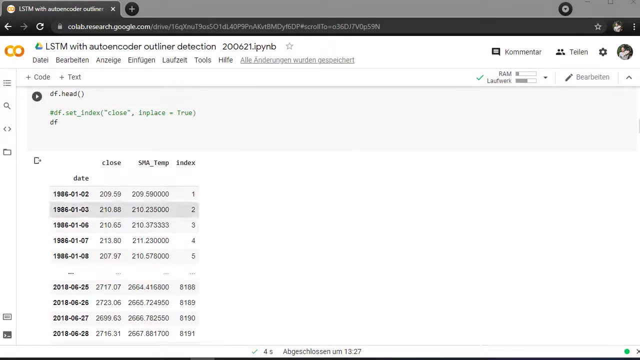 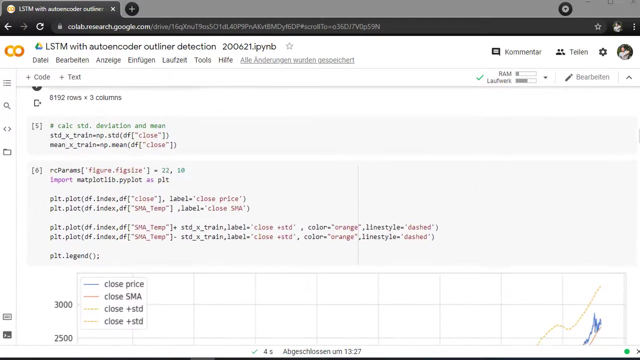 I downloaded the S&P 500 stock market course here from 88 to 2020.. And I just plot it here. I put date in the index, So you have the closing function And the mean average. due to time, I plot everything here. I was calculating the standard deviation, the mean and so on. 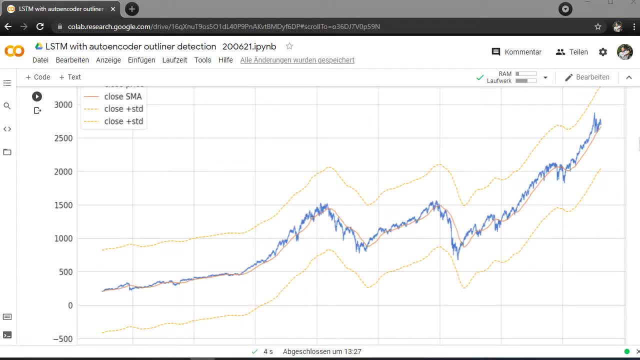 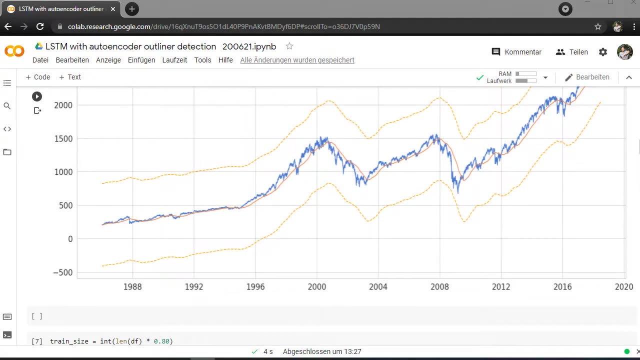 The mean is the red signal. here within the blue signal It's a little bit smooth, as you can see here. The yellow or the orange dot line or dashed line, here is the standard deviation Where you can see here and then you can already see. let's say: 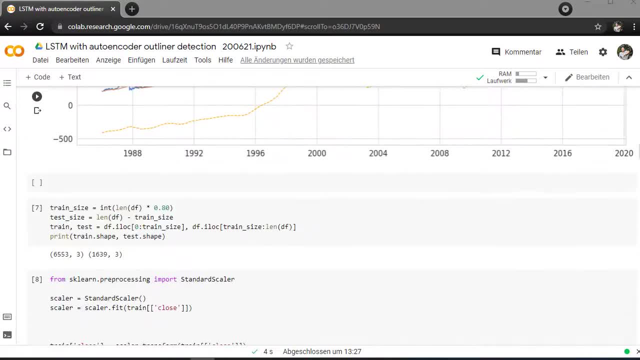 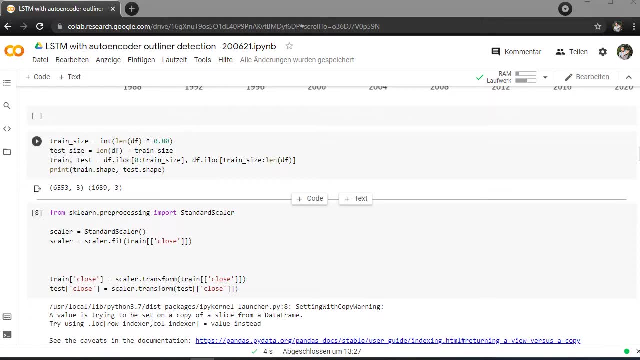 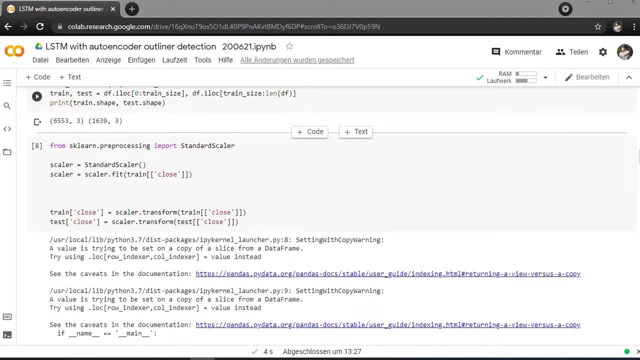 How the signal is going further. I split the training set 80%, test set 20% And afterwards I took the standard scalar here Standard to just transform the signal within 0 and 1.. It's better for the updating of the weight and calculating the weights. 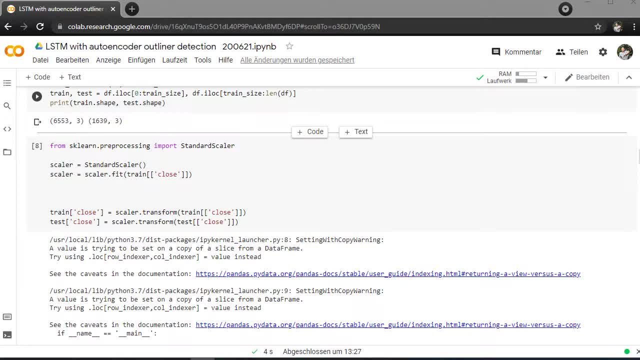 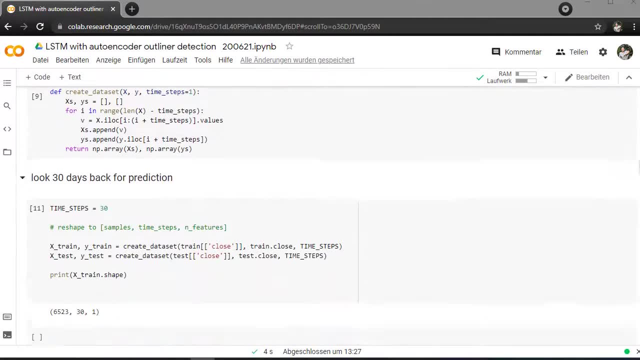 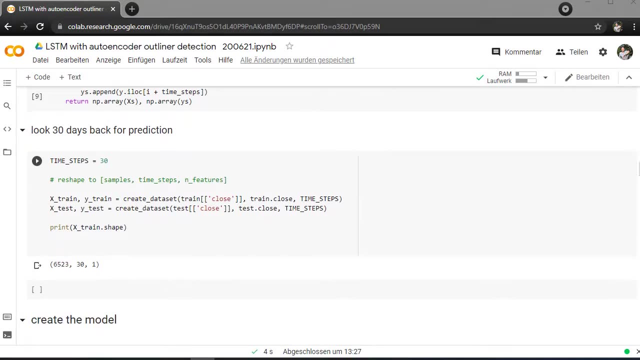 So I think this is really a nice thing That you always have to do within signal data. So the next thing I'm creating in the data set- Because I need this for the next function- To say that I want to look back at the last 30 days. 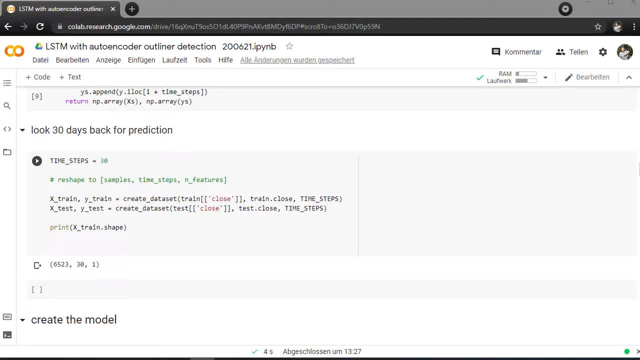 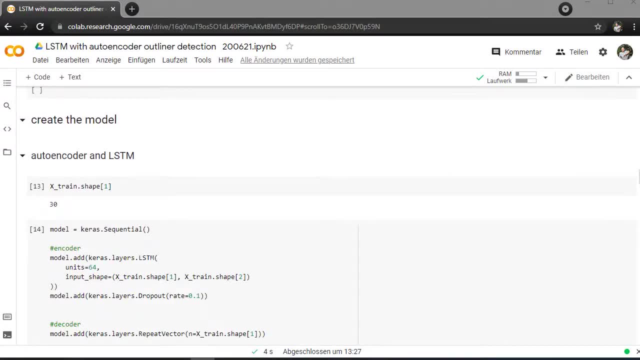 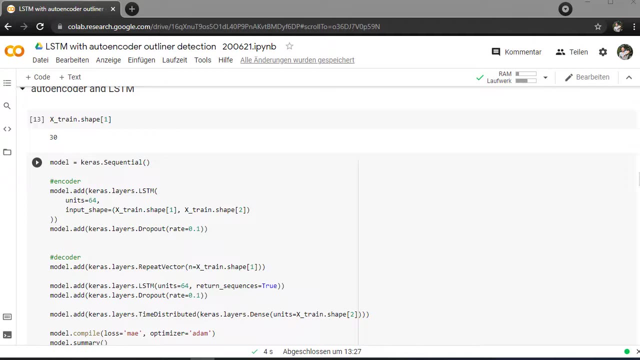 So I'm looking back at the closing course minus 30 days To calculate the prediction For the next step. So, as I already mentioned above, This is the model here, a sequential model. Start with LSTMs, 64 neurons and dropout rate 10%. 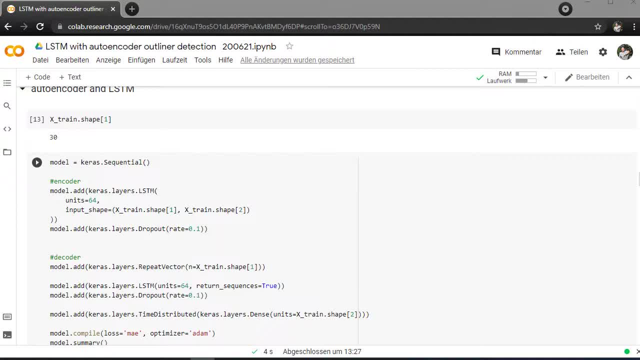 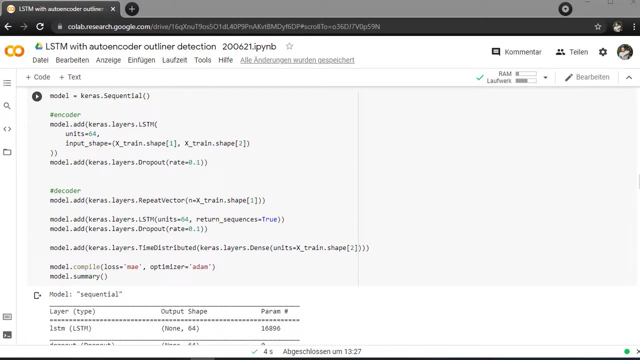 So each 10% of the connections will be dropped Due to not having overfitting. In the middle we have the repeat vector- It will be repeated- And another LSTM And time distribution. at the very end I have the ATEM optimizer. 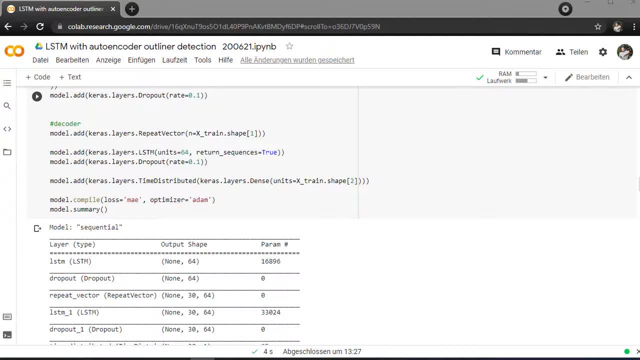 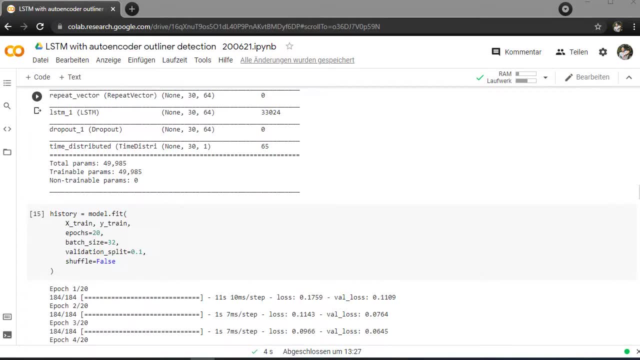 And the loss is the mean absolute error here, Because we are doing basically a regression here. So no accuracy, only a loss. So I have almost 50,000 parameters, Or let's say almost 50,000 weights, that were updated. 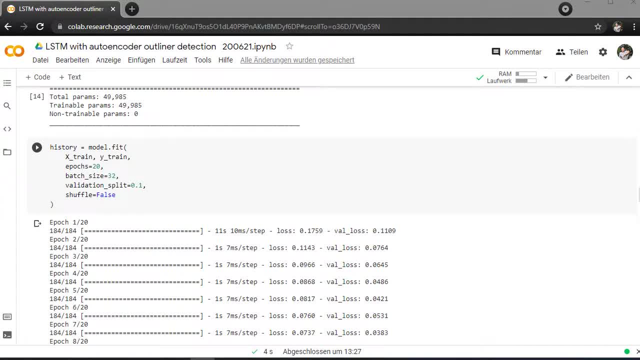 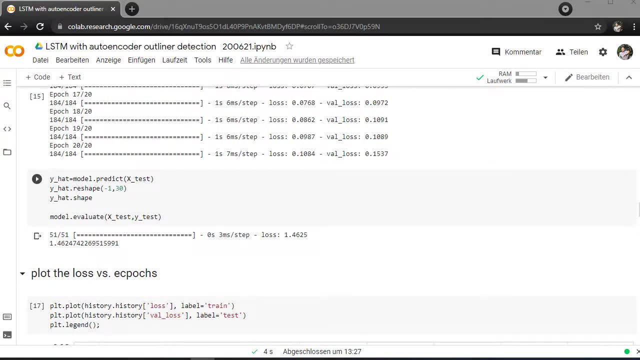 And I only inserted to training the model 20 epochs Shuffle false because it's a signal here I don't want to have any shuffle. It's no classification, So I put shuffle on false. After training the model you can see basically that the loss is pretty low. 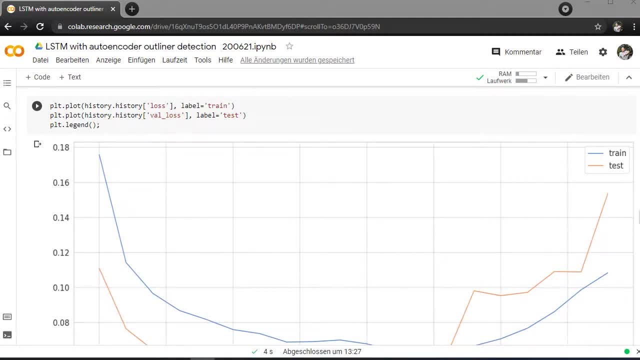 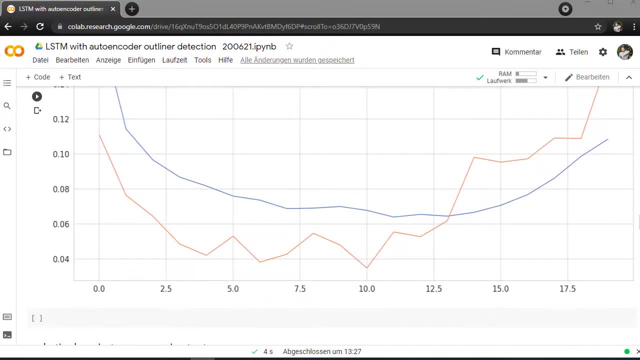 Here I plot the loss and the validation loss. The training loss is the blue line here And the validation loss is the yellow or orange line here. It's going already up after 10 epochs, Which shows us that this is the overfitting here. 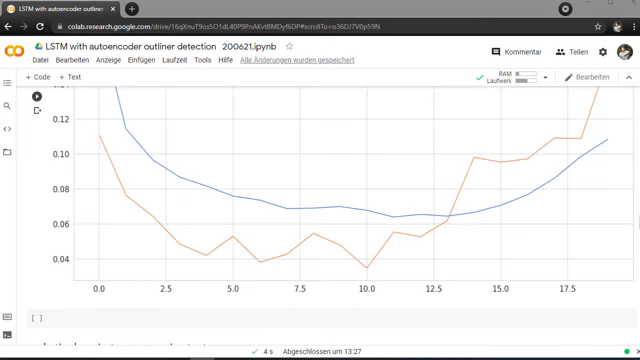 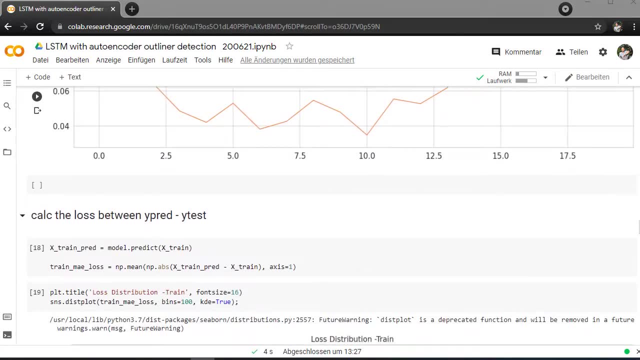 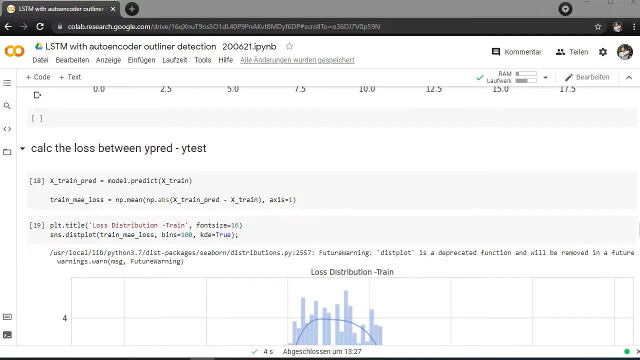 So you don't need so much epochs here. I would recommend only 10.. But I just want to show you in this example how you can do it. So I was calculating the loss between the prediction and the testing signal And signal data here. 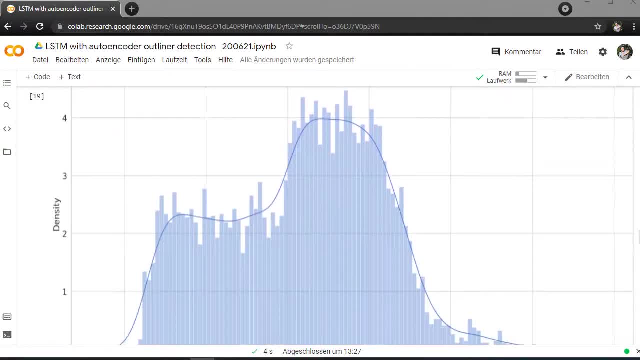 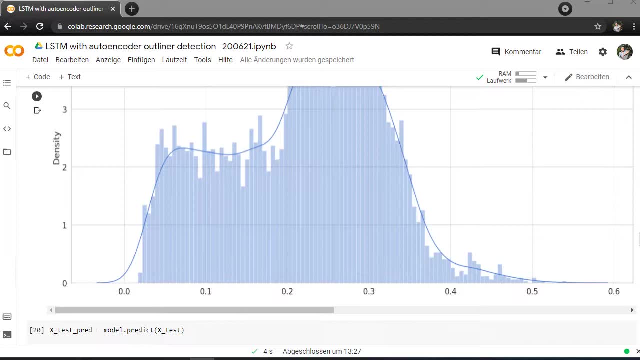 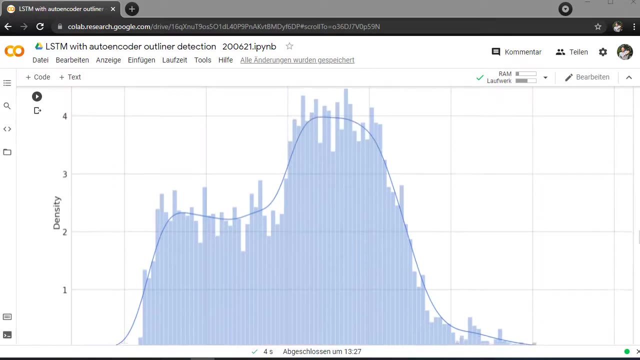 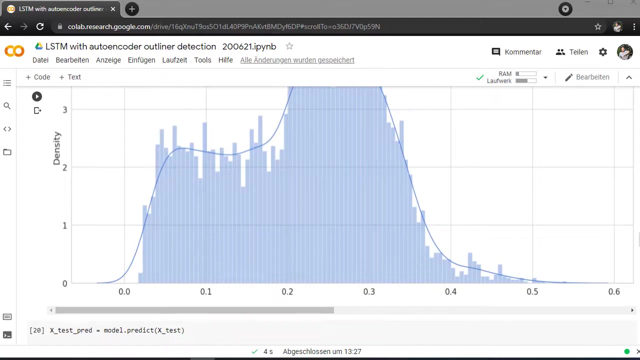 And plot the loss distribution. And you can see the loss distribution here. Just counting the number of the deviations or the loss due to the train data We have here, the most times We have 0.2 or 0.3 loss. 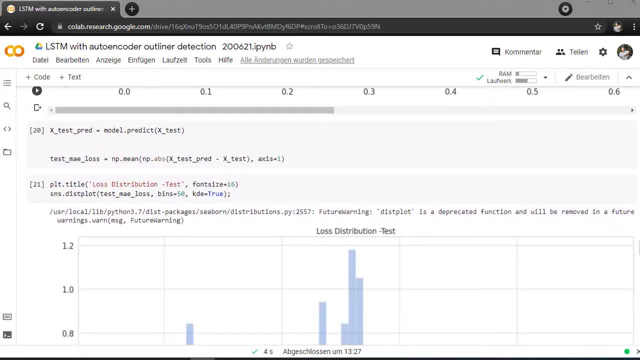 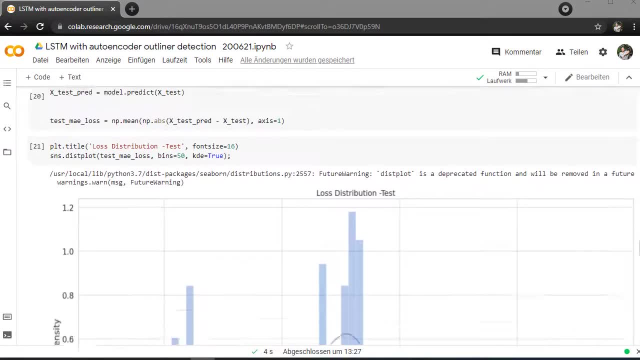 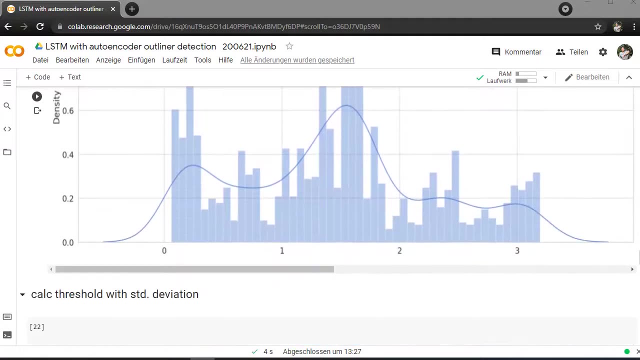 And if you are doing the same at the test data and compare it, Then you can really see that this is much more Higher. So there is a deviation or loss between 1 and 2. Which is the most significant one of the loss distribution. 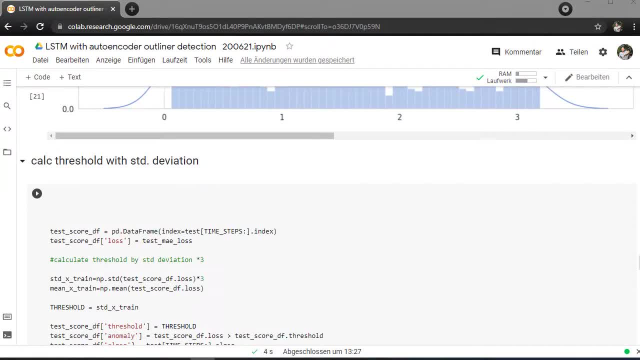 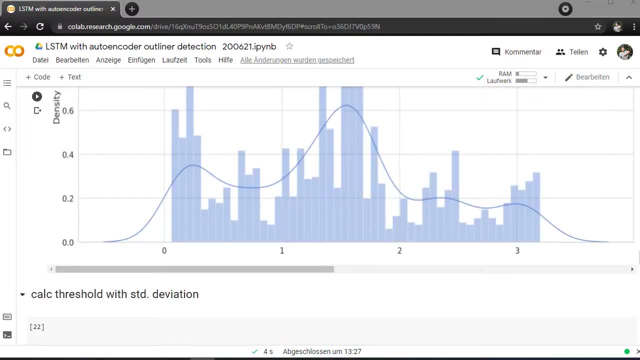 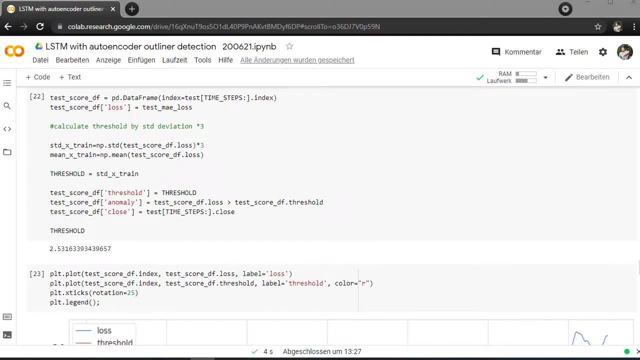 But now we are concentrating on the test data. here I want to calculate the threshold. here. I can say: okay, it's between 2 and 3.. Where after this only outliners are coming. So if the loss is much more higher, 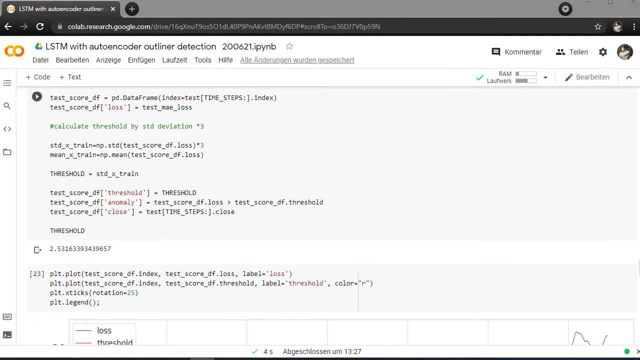 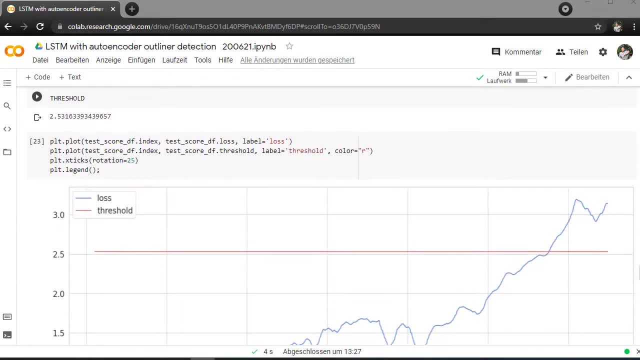 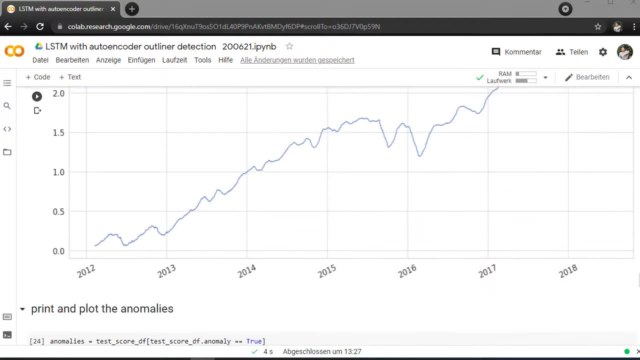 Then it's an outliner basically. But I calculate it just basically with the standard deviation here And it's 2.5.. And I also plotted it here: The S&P 500 threshold: 2.5 over loss. So if you are printing this, anomalies that we are detecting here. 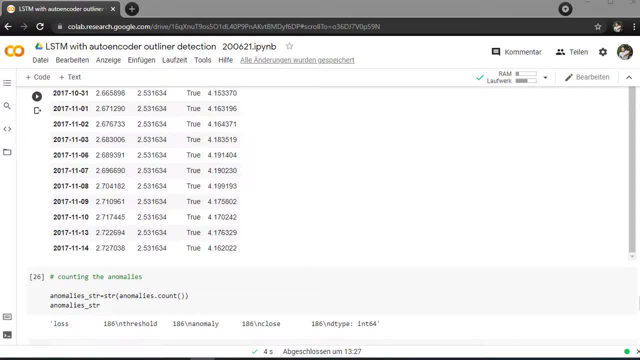 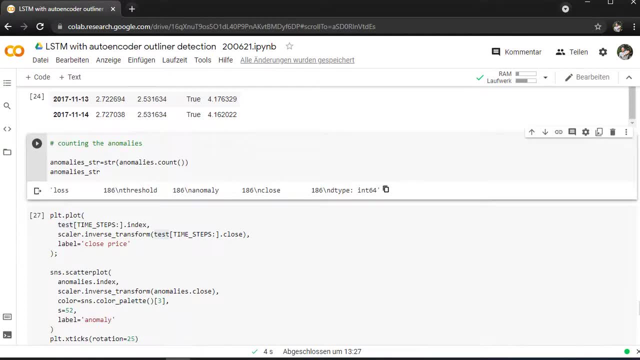 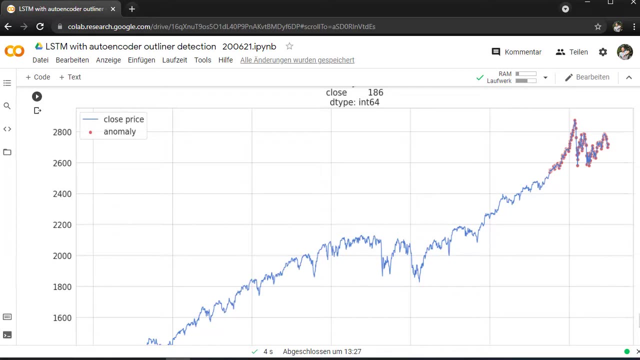 You can see in which date it was calculating and detecting. We have 186 anomalies here And if you are just plotting the 186 anomalies which are red here- Red dots, You can see that basically up from 2018.. There is a lot of rapidly increasing here. 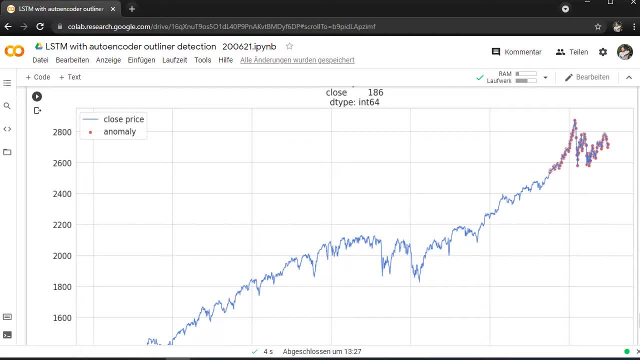 And rapidly decreasing. So there is something going on here And you can basically find the anomalies here. You can also play around with the threshold To make it even more sensitive, But that's my recommendation. You can play around a little bit. 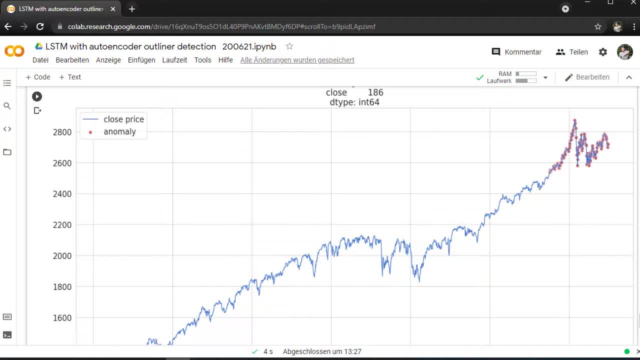 To find the best fit for your project. So thanks a lot And hopefully, if you like this content, Hit the subscribe button And see you soon.